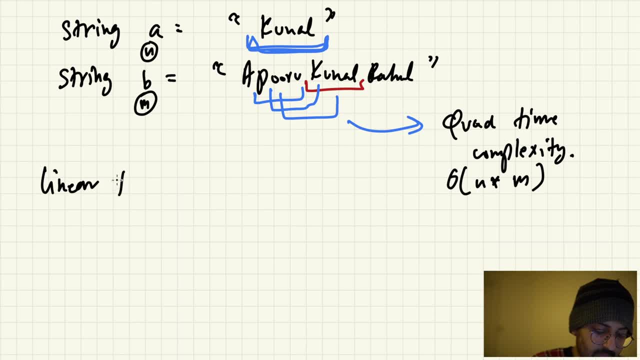 M quadratic. Can you do it in linear time? O of N plus M, for example, Can you do it in linear time? How can we do it in linear time? That is the question. That is the question. For that we're going to use hashing, We're going to use hashing. So this is a popular 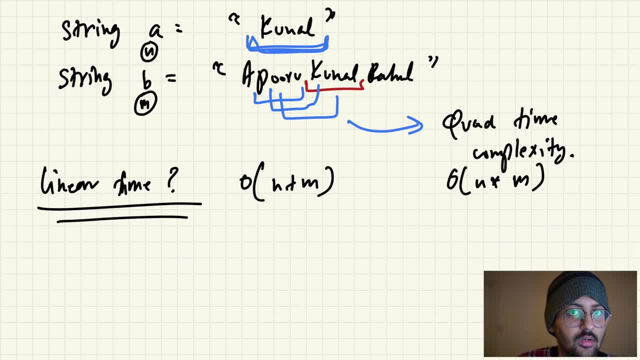 algorithm It's like used. for example, if you want to talk about Google search, Okay, So ideally you can say somewhere there hashing is used when you try to search for items, because you know Google search has its like database and it has some like. 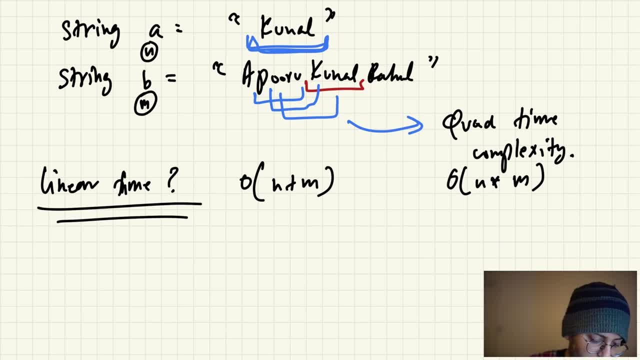 pre-stored values and stuff, And the algorithm in this video, very important one for string searching in linear time. I hope you understand the question right. Linear time we're going to use is called Karp-Rabin algorithm. It's very simple: Rabin. 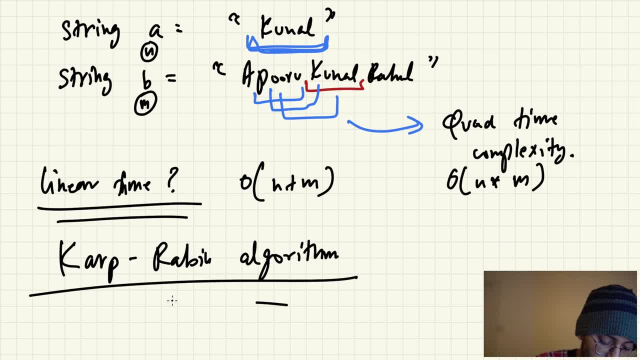 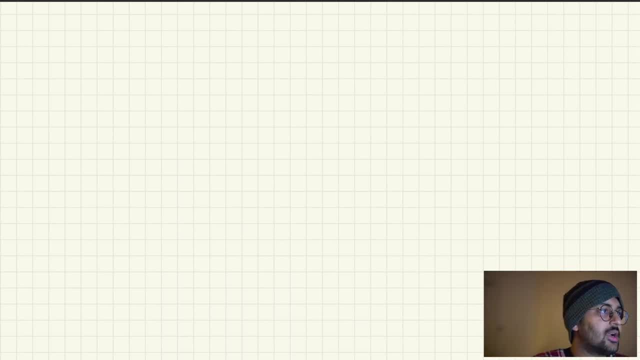 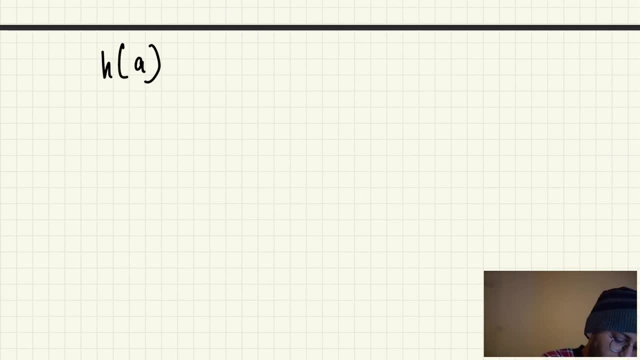 algorithm is something we will learn today, So we'll obviously look at the theory first, then we'll look at the code. So what Karp-Rabin does, is that what it does is it compares the hash value of A. It compares the hash value of A. 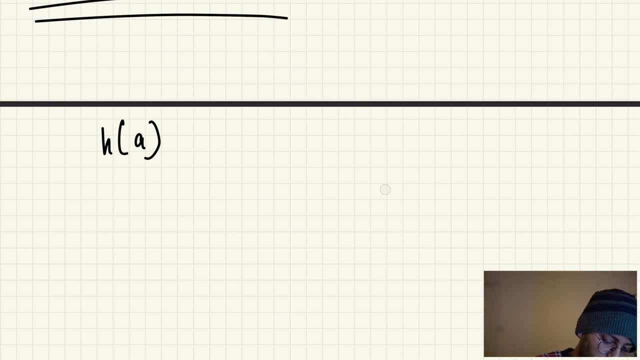 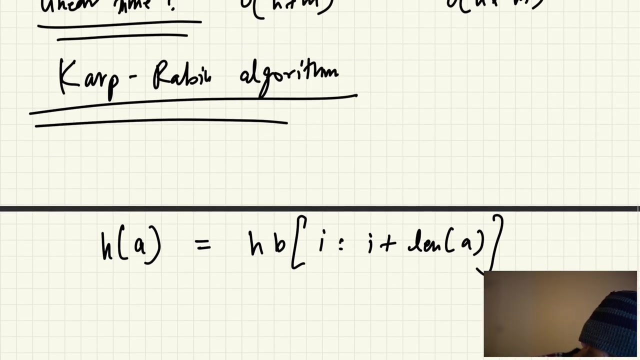 In string B. so it will compare the hash value of what Hash value of B, but not the entire B, from I till I, plus length of A. And this is very simple. There's nothing wrong with this. Why? Because if I have, let's say if I have, A is equal to K U N A L, 0,, 1,, 2,, 3,, 4.. 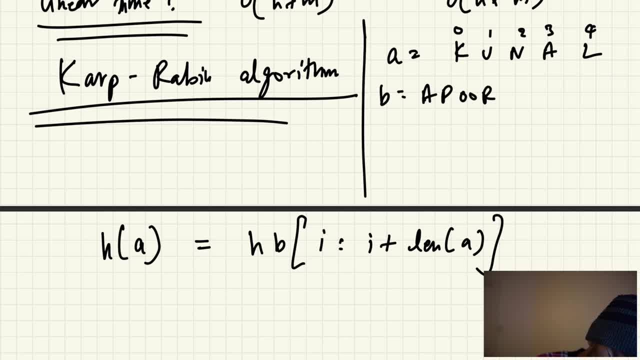 B is equal to A P O O R V K U N A L? R, So 0,, 1,, 2,, 3,, 4,, 5,, 6,, 7,, 8,, 9,, 10,. 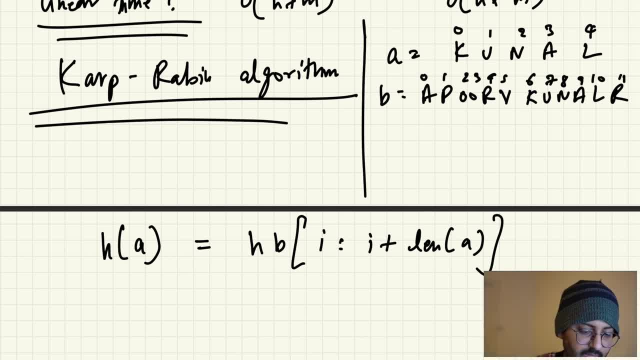 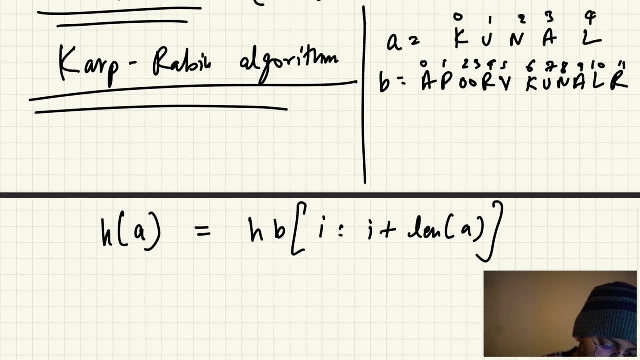 11. So it will compare the hash value of A, which is the entire thing, to the hash value of slots, To the hash value of slots. So first slot of size 5 will be this, Then the next slot of size 5 will be this, Then the next slot of size 5 will be this, So on. 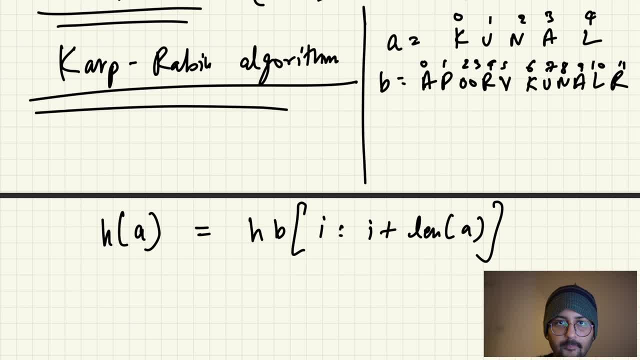 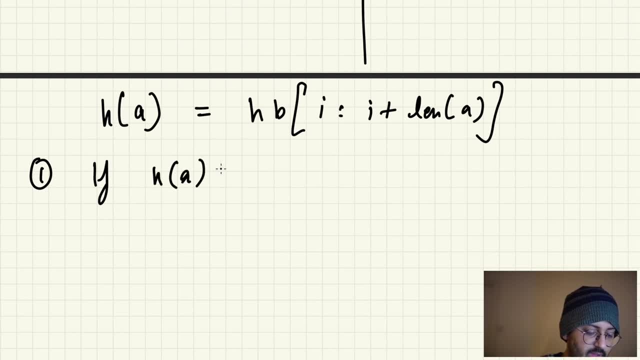 and so forth. Whatever you want to consider, I hope you are able to understand what I'm doing here. Okay, Because why are we comparing the hash? If hash of A is equal to hash of, you know, B, I till I, plus length of A, it might be. 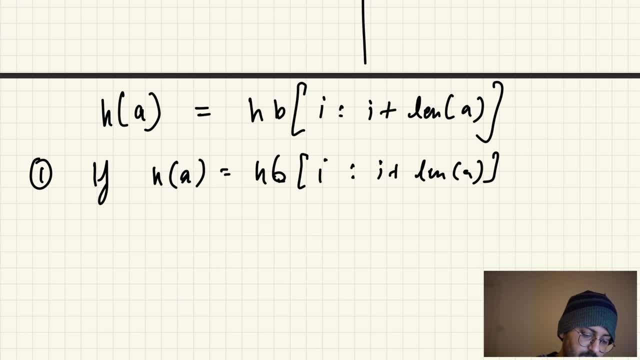 possible that match has found. Maybe found a match Because we know that the same item, the same string will have the same hash map. Sorry, same string will have the same hash value. Hash value of Kunal will be equal to hash value of Kunal. only, like all the time, Right. 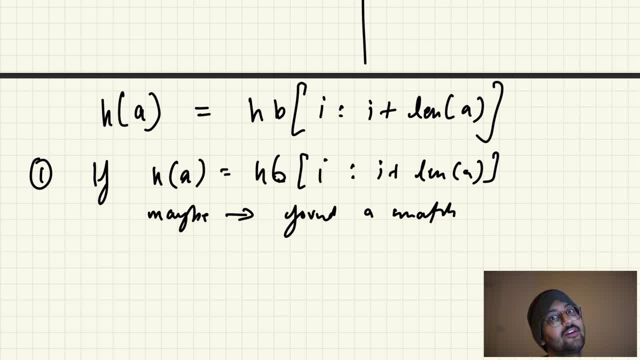 What are we going to do? But also we know that multiple strings can have the same hash value. It might be possible the hash value of Kunal and hash value of Rahul is the same number. That can also be possible Because in the end it's just an algorithm. Okay. 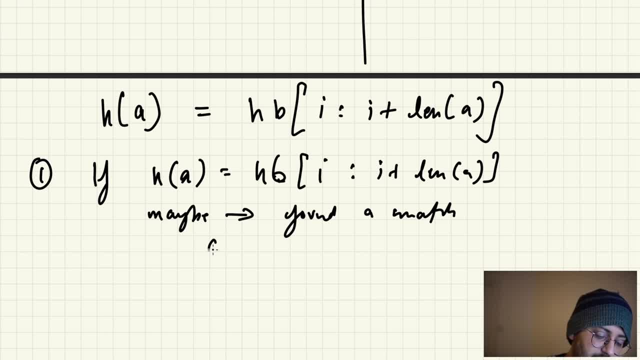 But the probability of that is less. So if you have found a match check. And then, if you have found a match check, Every character. Okay, This is going to take O of A time, Because every character in A 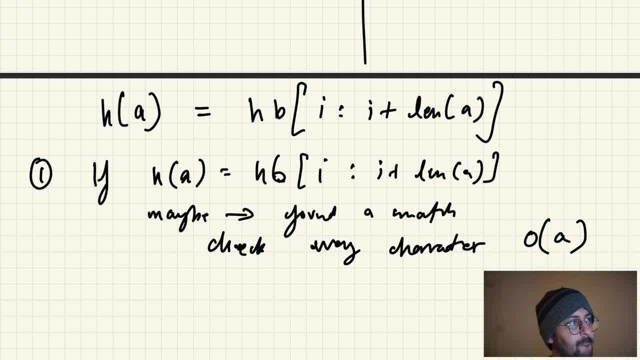 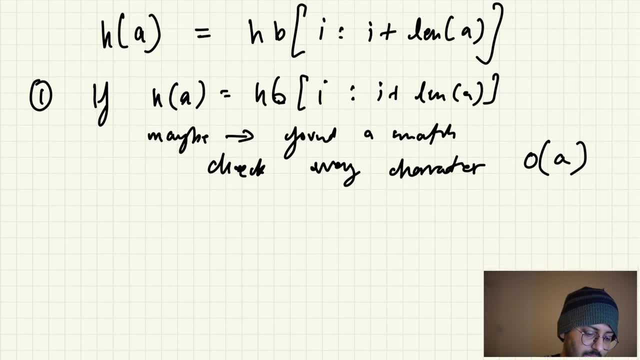 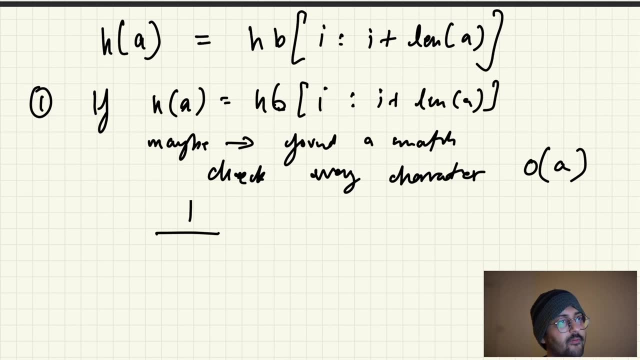 I will check with the subset that I have found. Okay, Problem solved. But if you have not found a hash value like this, if it is not equal, you know, then it happened with a probability of one upon 1. Okay, 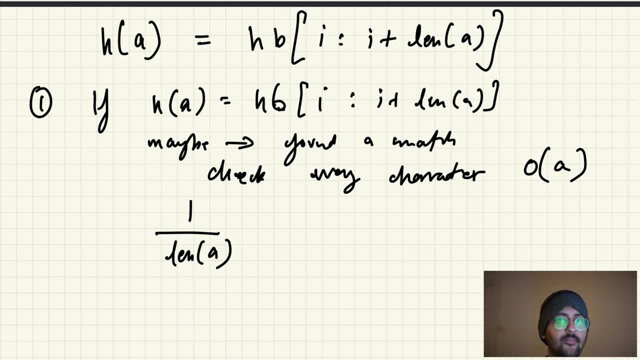 What Length of A, How? Previous lecture, the section was universal hashing. We covered this in detail, so check that out. If not, then that was the probability of it not happening. Okay, If not, what? If not, let's say, for example: I'll write it down again. I know you're confused, So I'll write it down in steps. If you find a subset in B which hash value is equal to hash value of A, then maybe you have found a match. So you will check for every character. 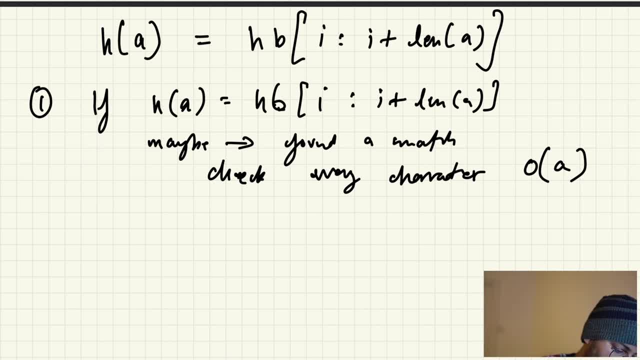 So 0.1.. Maybe you have found a match and you will star star. You will check for every character. If all characters equal, then I have found my answer. But let's say there was a scenario that not all cars are equal. 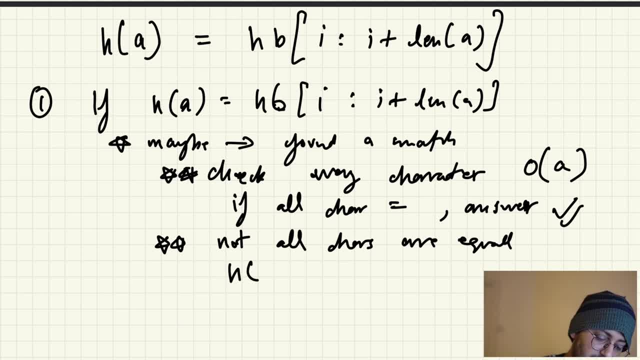 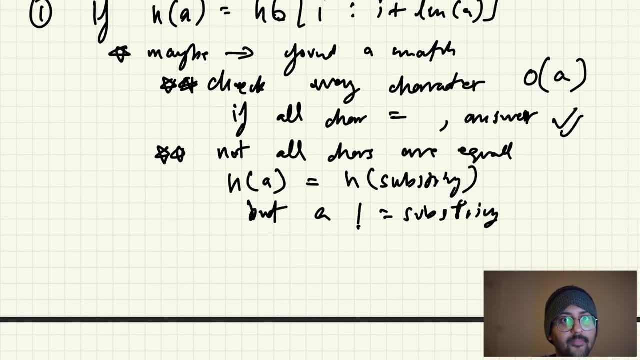 So hash map of A is equal to equal to hash function of A. hash code of A is equal to hash code of substring, But A is not equal to substring. Now you understand. So two strings you have found with same hash code, but the strings are itself different. So the probability of this happening is what? 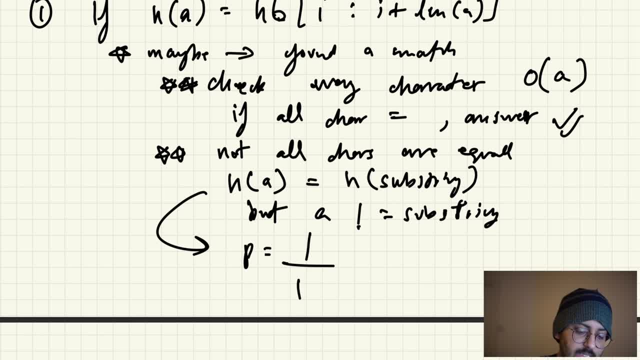 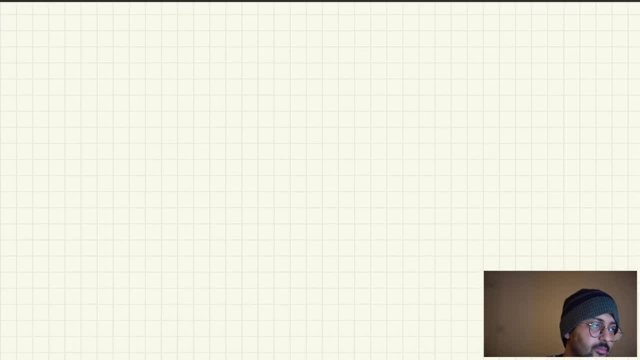 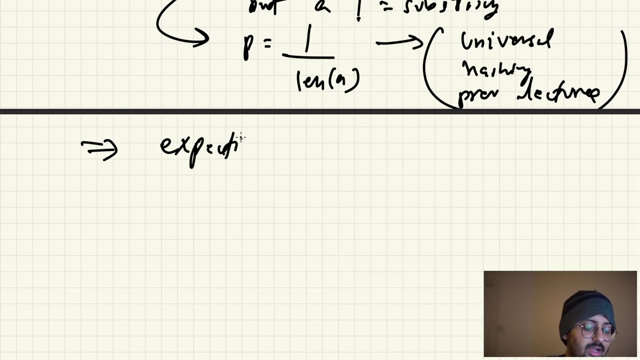 Probability of this thing happening is 1 upon size of A. This can be found in universal hashing in previous lecture. Now you understand, Okay. Now I have mentioned it in steps, So I hope you understand now, Okay. So expected cost or amortized cost, Expected cost of every I. 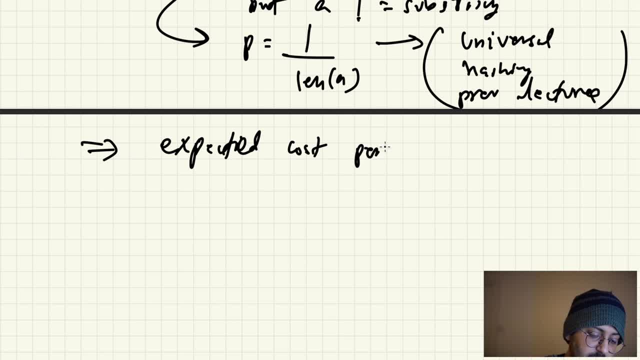 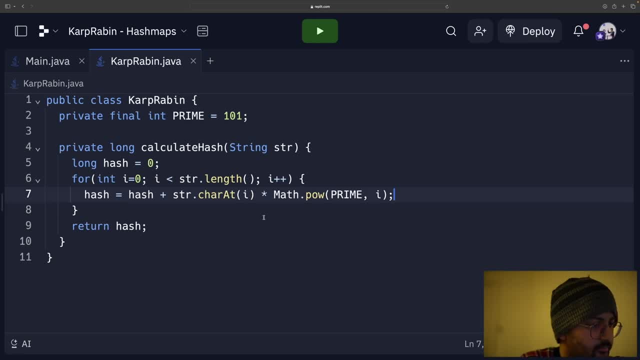 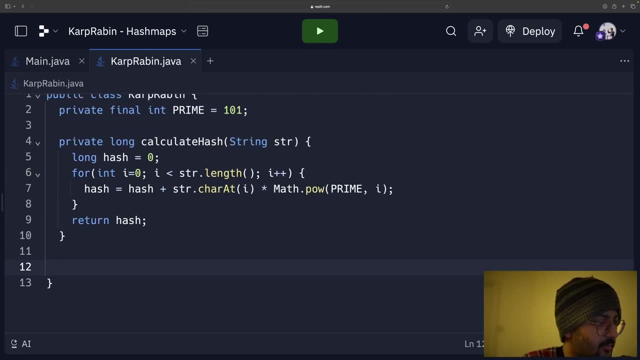 Okay, Just a simple function that I am doing. Okay, Just a simple function that I am doing. So this will give me the hash value. Okay, But now let's say what I am doing is I am going to a new window. 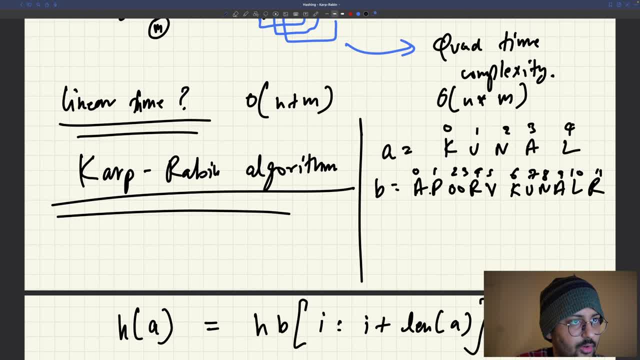 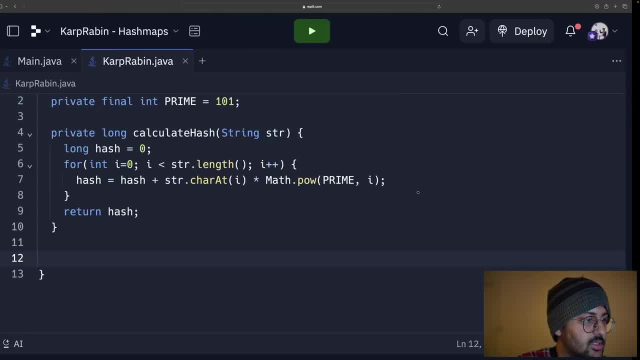 So let's say, first I was calculating hash for this, but now I am like: okay, I want to calculate hash for the next one. So V is added and A is removed. So for example, I can say private. 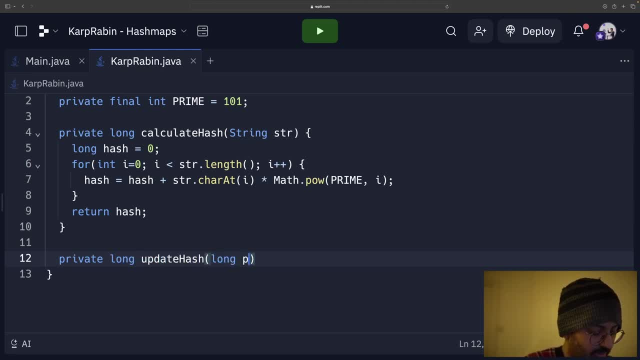 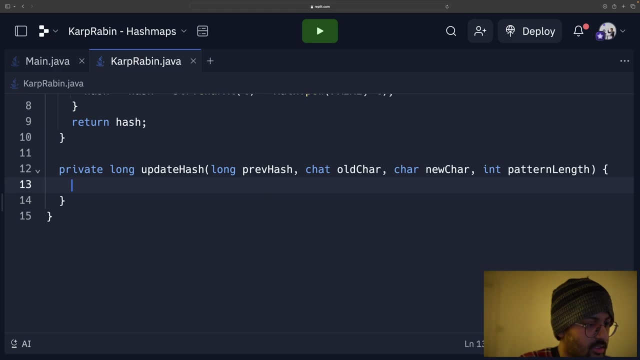 long up date hash. I will give it the previous hash value, I will give it the old character, I will give it the new character and I will give it the pattern length. okay, I'm going to give it the length. so the pattern that we are searching for. so previous hash. so this a I have to remove first. 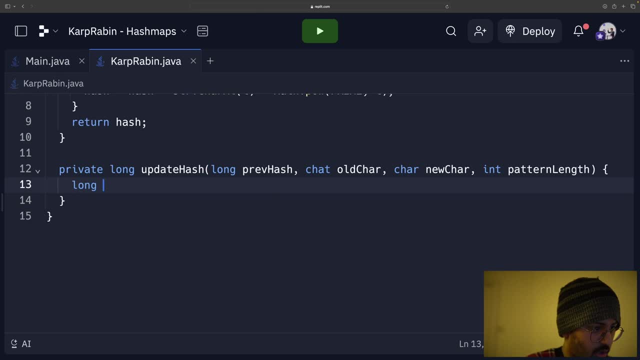 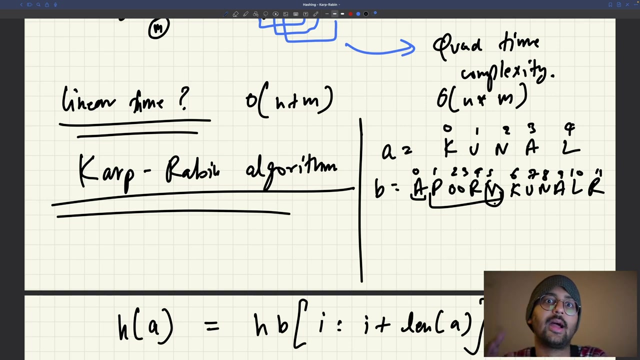 okay, I will remove a. I'm going to say long. new hash is equal to previous hash minus old character. divide by prime number. okay, add in the new character, so you can see. now I'm not calculating the entire hash again, this is called rolling hash. in constant time I can find the hash value of p o o r v. 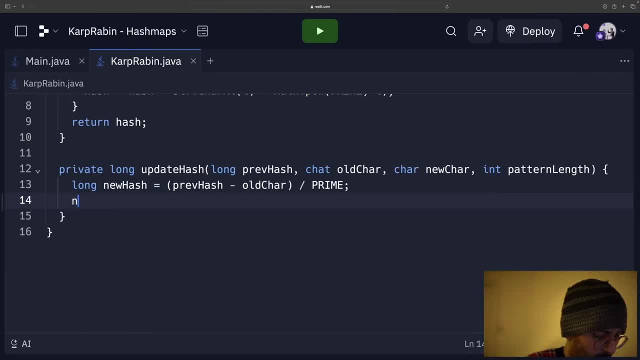 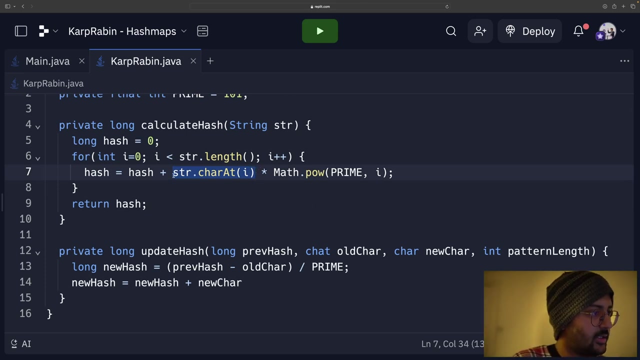 because I removed a and I'm adding v. so adding v new hash is equal to new hash. plus what new character? same thing, new character, right. so here we have a new character multiplied by math dot power of prime and the index it is at: uh, what is the index? i index. 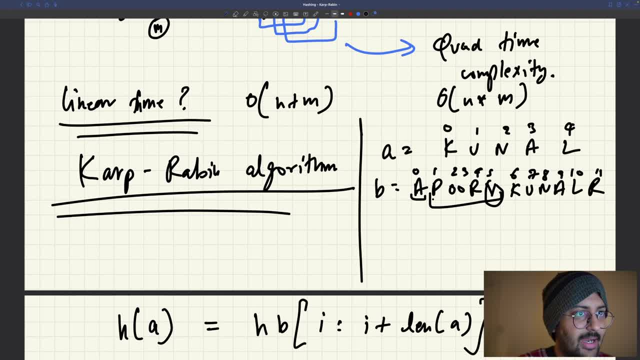 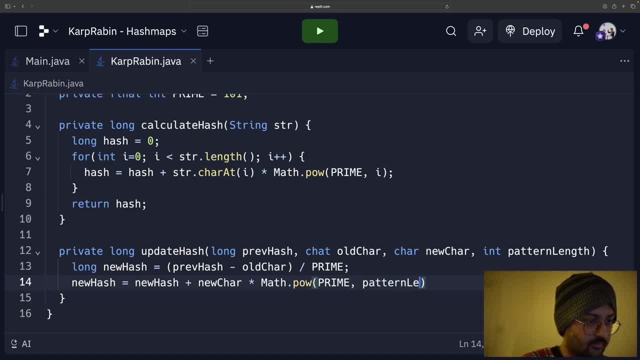 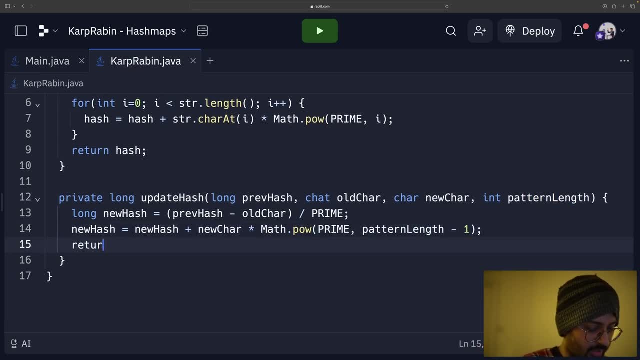 i will be equal to what the pattern length minus 1. you can do a dry running return new hash that I have already left off. let me run, run after it, see if I can change it. so I've made a new sandals the first. i ordered x as new hash. aftermış. our hash is clearly misrepresented by the p o o r v. this is a very good way to solve. mission statement in the review. when you run new hash, you have to just run that into a dry running run. that way you don't have to go to através. now let's close, i walk. 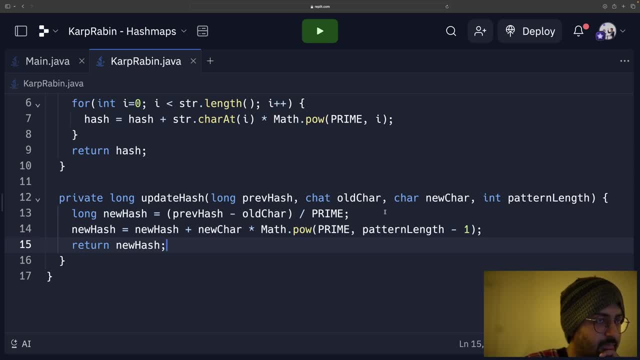 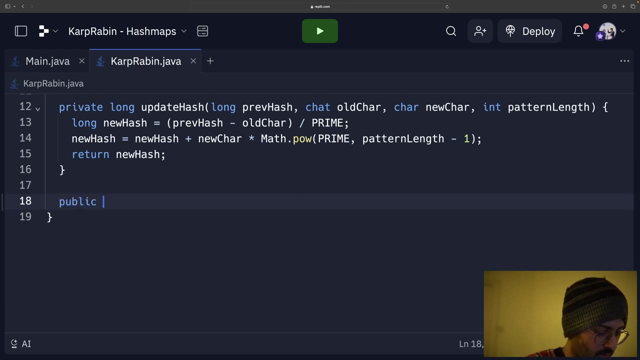 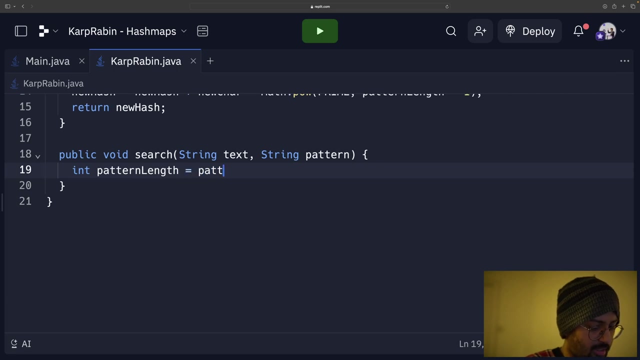 open. I return a new hash i x from the phải windows, the path. now that's all. and now let's looks good, that looks nice. okay, next up now the carpet ribbon algorithm. so public void search for. in the string text. i want to search for a pattern. okay, so my pattern length. i'm just going to take pattern dot length. 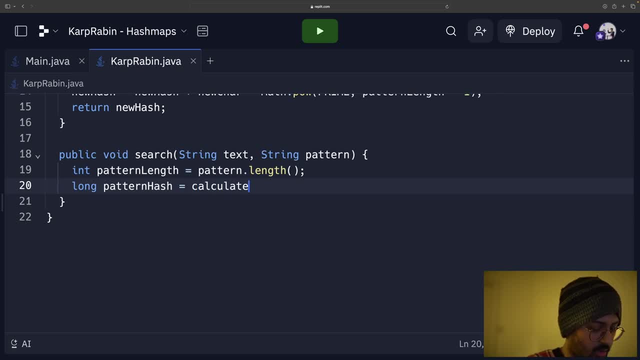 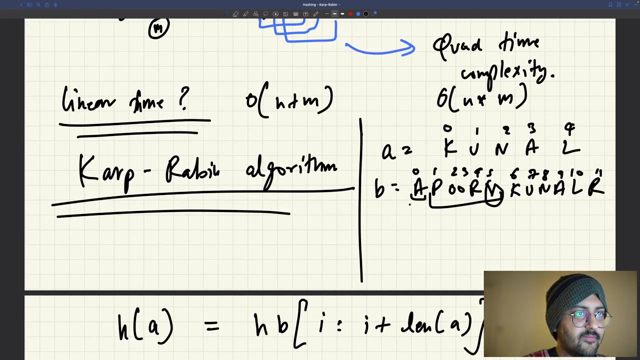 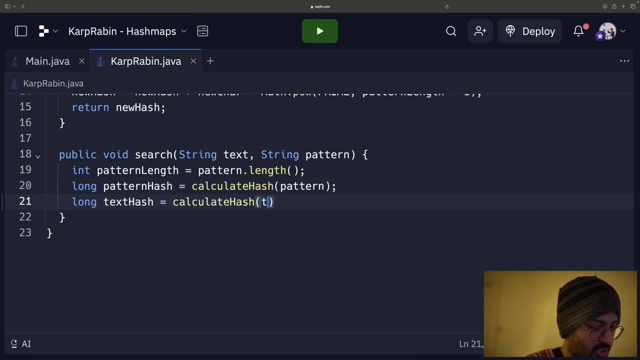 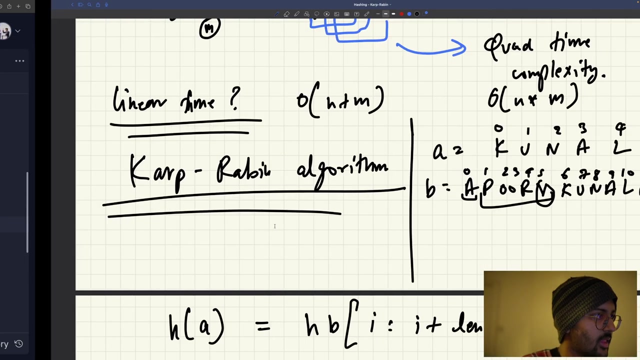 pattern hash. i'm going to take calculate hash value of pattern my text hash. i'm going to take initial the first sub array of the size of my pattern calculate hash text dot sub string: zero pattern length. okay, sounds good. what are we going to do now? i'm going to check for the for every window. i will check. 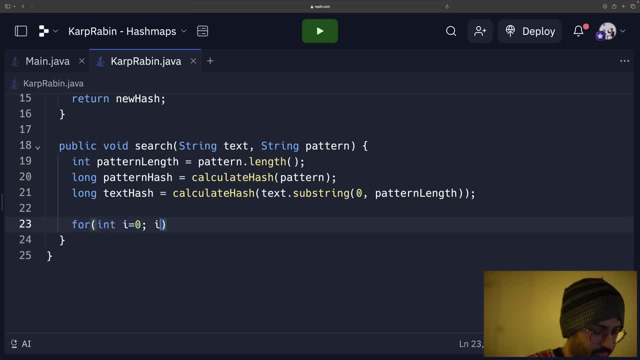 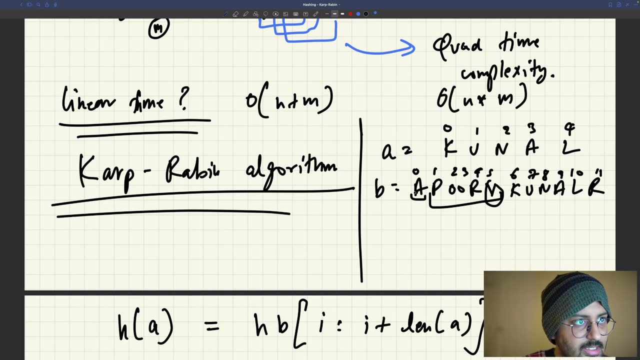 so for int i is equal to zero. i is less than equal to what the overall text dot length. but since i'm taking windows, if i take, for example, i is equal to 9 over here, then 9 plus pattern length, you can see it's going out of bounds. so maximum i i can go to is 1, 2, 3, 4, 5.. 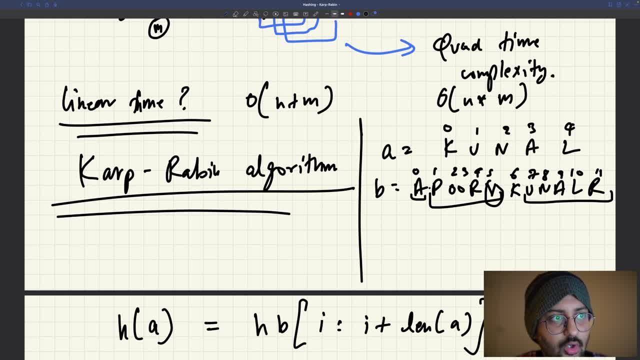 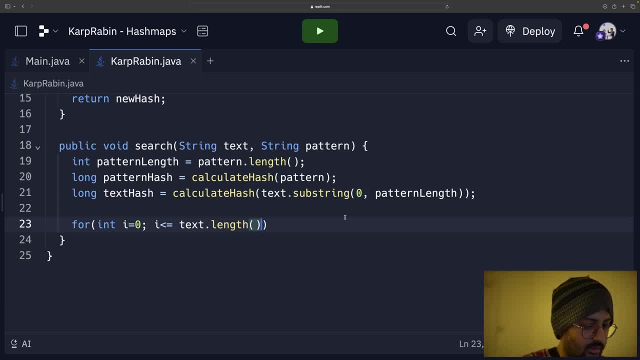 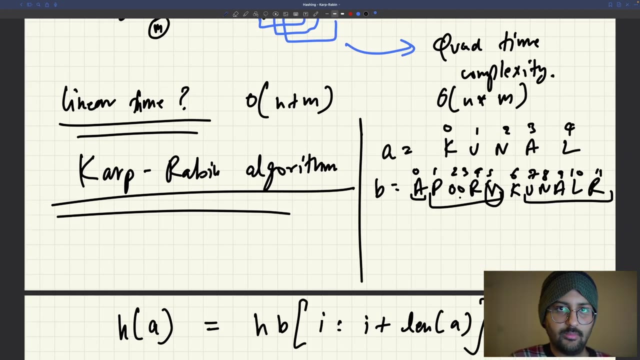 this is the maximum i i can have at 7. so total length minus the pattern length. so i is less than text dot length minus the pattern length. okay, sounds good, and i plus plus. this is how we have our window. this is also like sliding window problem, okay. so just because understand right, if i take i is equal to 9 and i say 9 plus. 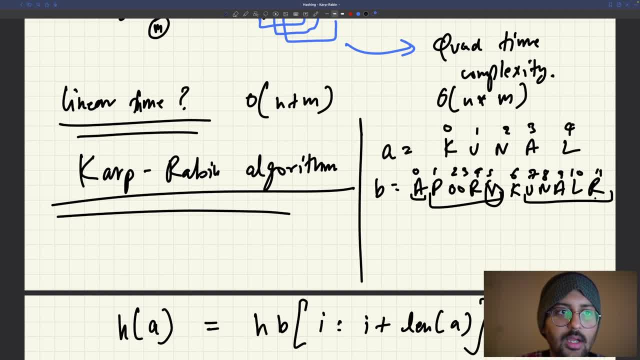 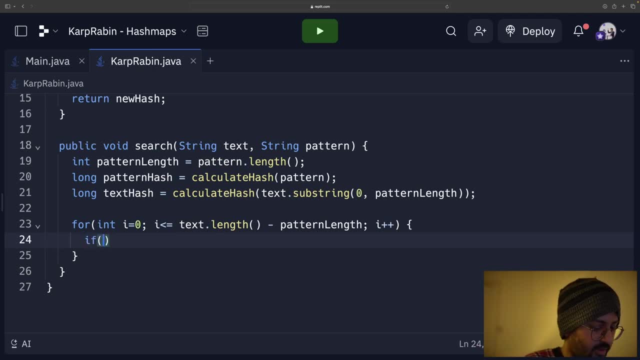 9 plus length of 5, that will go out of bound maximum. last, what is the last sub array? i will sub substring. i will have this one. what is the start index of that total length minus the size? okay, now i will check if text dot substring of. 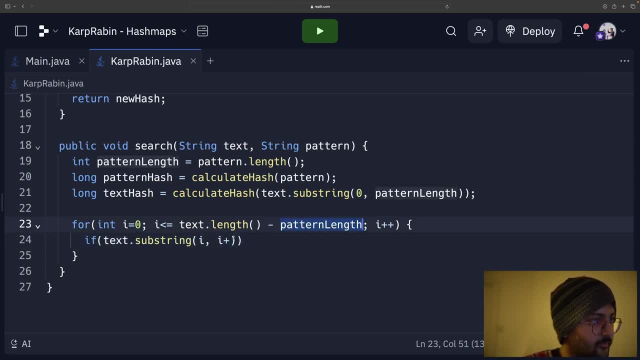 i till i, plus pattern length is equal to my pattern. i will check this when. if the string is equal, if the hash is equal, if text hash is equal to equal to pattern hash, i will check if these strings are equal. if yes, i can say system dot. 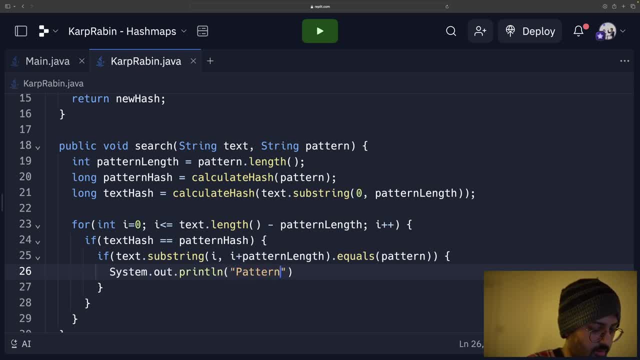 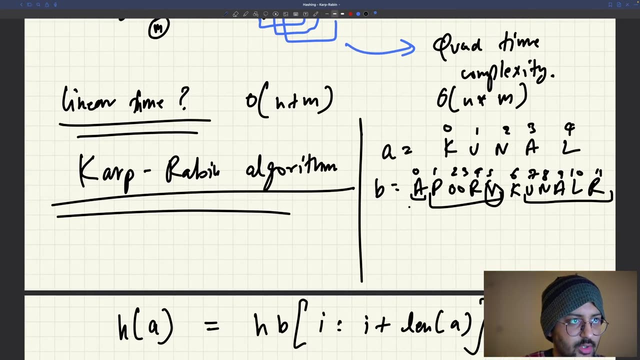 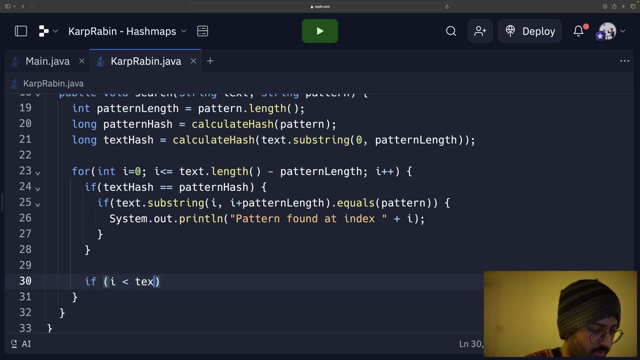 dot print l n pattern. found that index i okay. otherwise, if this is not working, this window is not working, i will move ahead by one. so i will move ahead by one, i can say if first of all i'll do a check before moving ahead by one. 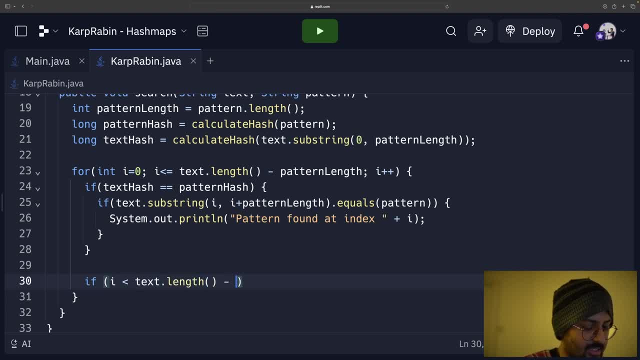 if text dot length, if i, is less than text dot length minus pattern length- because i don't want to go out of bound- it's the same thing- then i will update the hash. so new text hash is going to be equal to update hash function. i will pass in my text hash the first character that i'm removing: text cat. 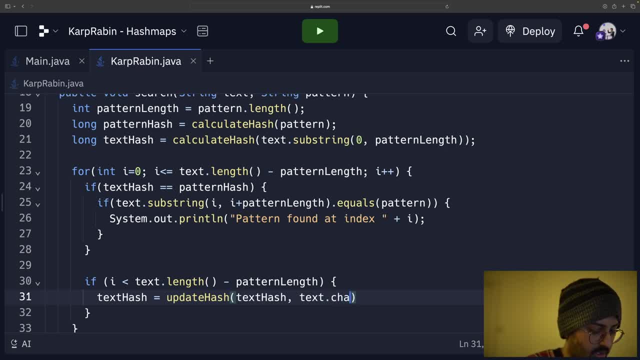 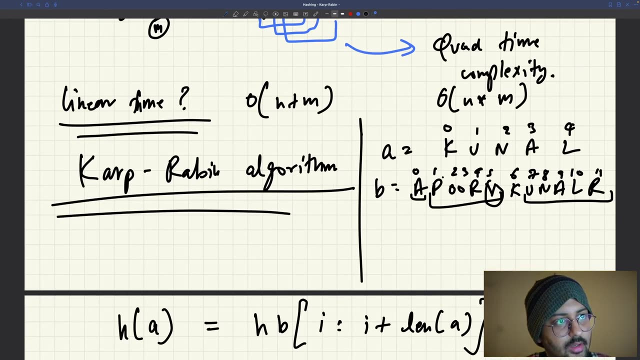 at text dot care, at i, the next character, which will be text dot care, at i. the next character i plus pattern length. because, think about it, the first character will be the character i and the next character will be i plus pattern length. so moving forward, okay, the next character here. 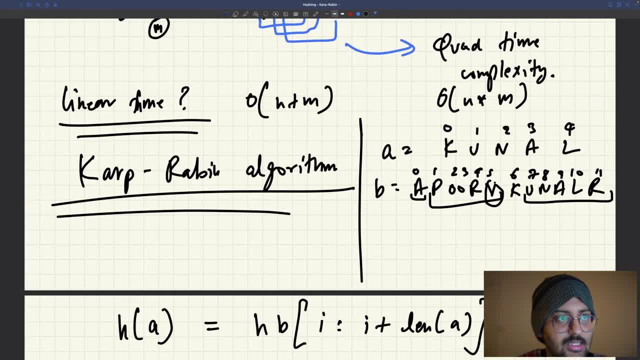 v, for example. so zero plus five, which is five. yes, that's the new one. i hope you're able to understand. you know, if you dry run, i just showed you this a and b examples. for example, if i'm over here at p o o r v, then i will remove this one, which is i. 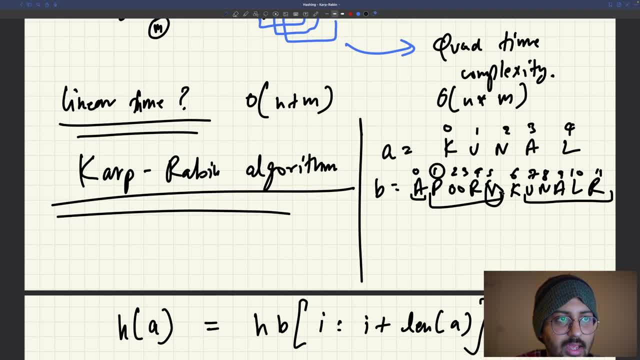 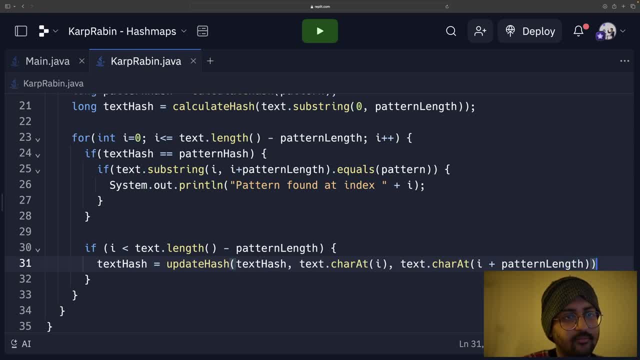 and the next one will be i plus one six. so yeah, k is the one i need to add. this is the one that i'll need to add. pattern length comma. i just need to pass the pattern length. that's it. that's it. that's the program. now i can run this. 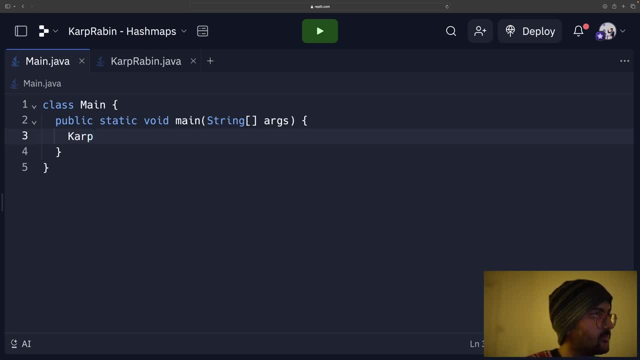 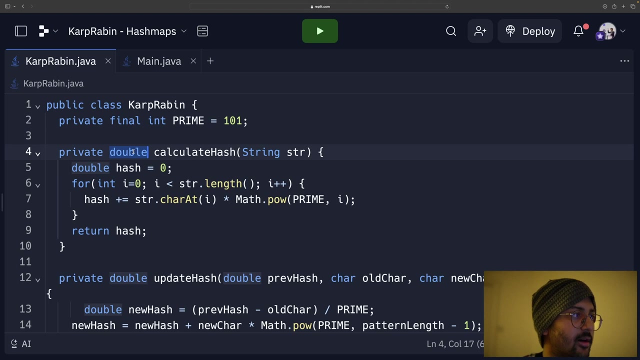 carp ribbon. algo is equal to new carp ribbon and i can say algo dot search. what do i want to search in in a poor kunal rahul? let's say i want to search for kunal. okay, one more thing i did. i'm storing the hash in double now instead of long, because this entire value was double. i don't want to.